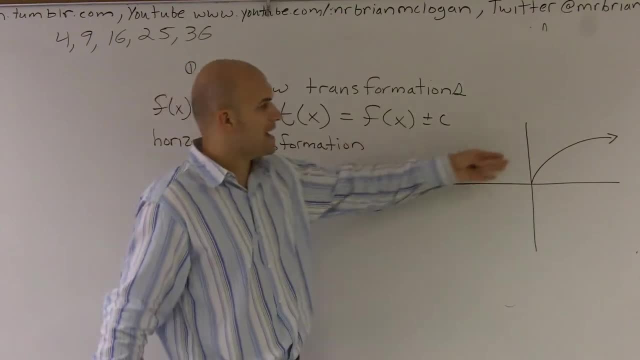 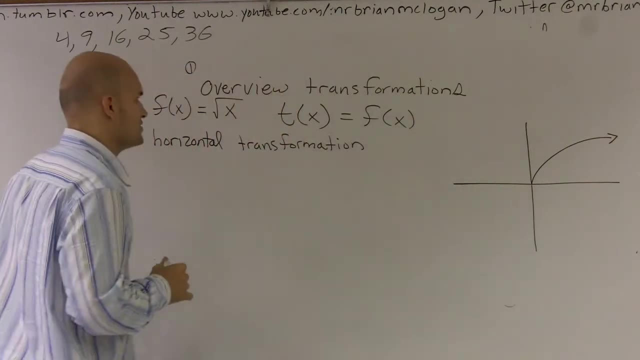 much a plus or minus c. Now, what you can think of what happened was that we shifted it up or down or changed the y coordinates. Well, now, what we're going to do is, when we're dealing with horizontal transformations, we're going to add c to our f of x. So when we're doing 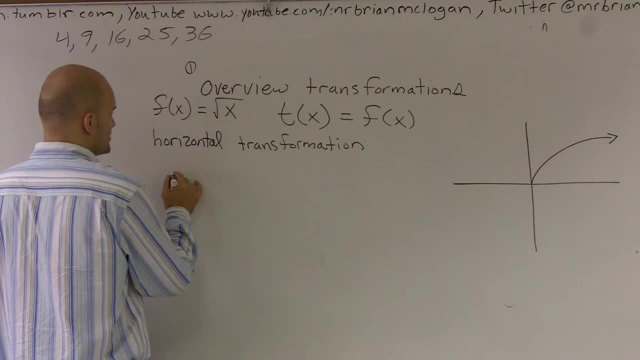 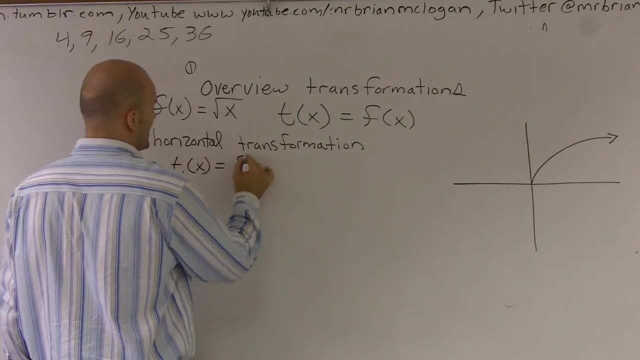 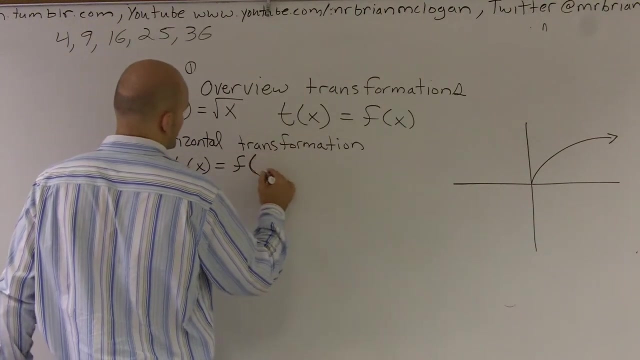 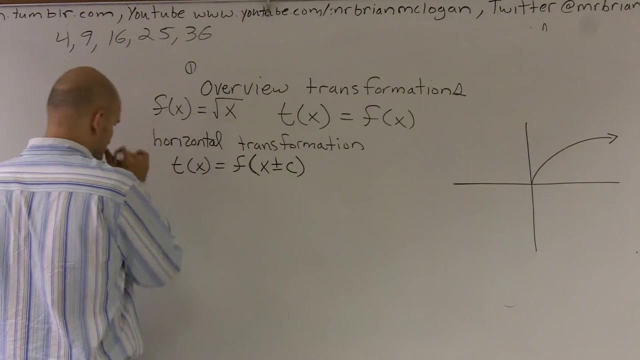 horizontal transformations. what we're going to have is a horizontal transformation. is now, when we do t of x is equal to f, and I don't know where to write this. okay, I'll just write. I'll just write x plus or minus c And we can just say when c is positive. 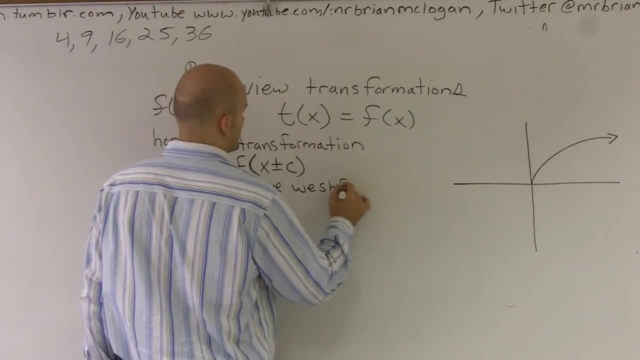 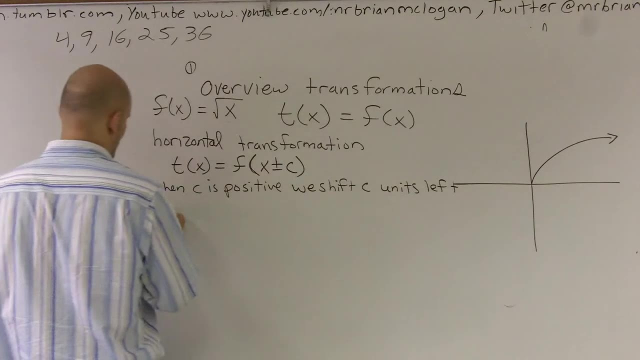 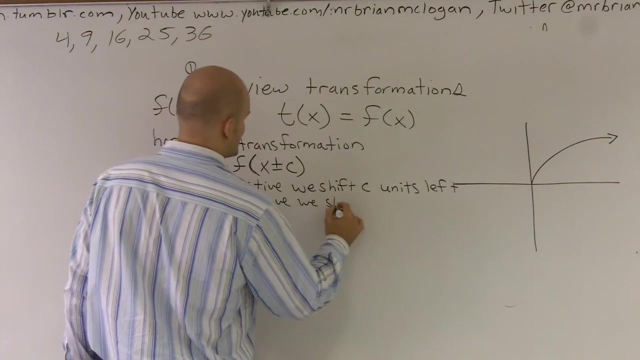 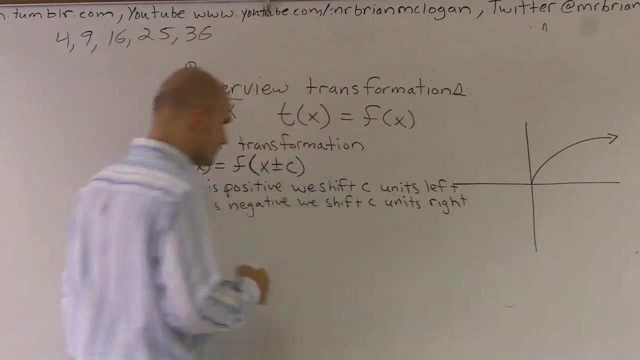 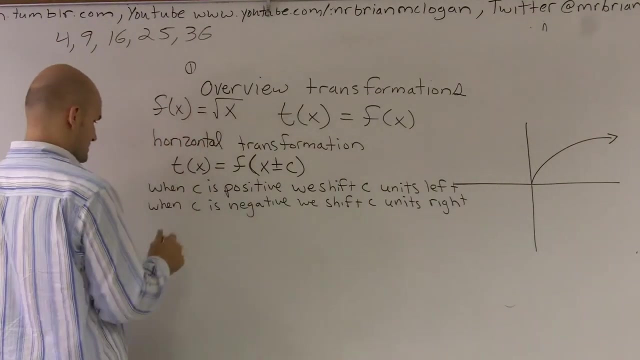 we shift c units left, And when c is negative we shift c units right. Now I'm going to give you a couple examples and then I'm going to kind of show you why that's true. So the first example: let's say, here's my f of x. So if I do, f of x equals the square root of x, and 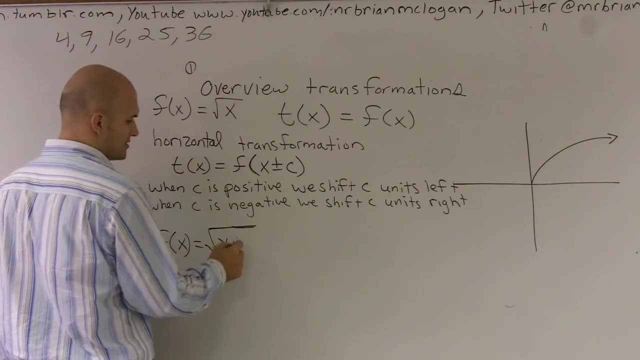 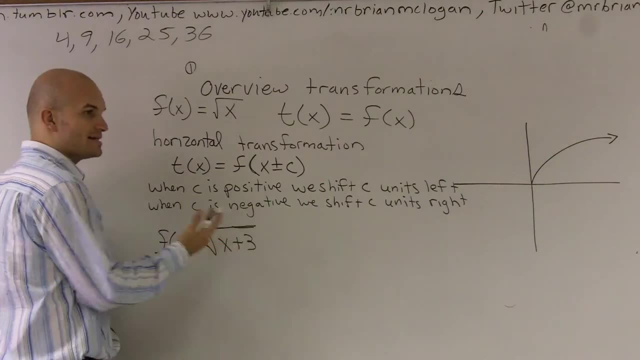 let's say it's now. now it's within my function, so it's going to be x plus 3.. So a very common mistake that a lot of students say. they want to say it's positive, so therefore it's going to go right on the Cartesian coordinates. so they say: you know, shift right 3.. But 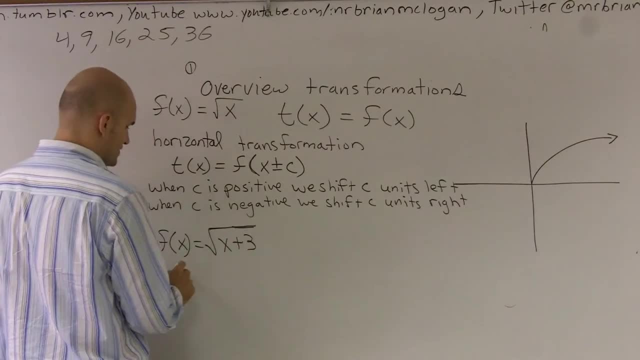 actually I'll show you in a second, but actually this is going to be shift left 3.. So what's going to happen is I'm going to shift right 3.. So I'm going to shift left 3.. So I'm going. 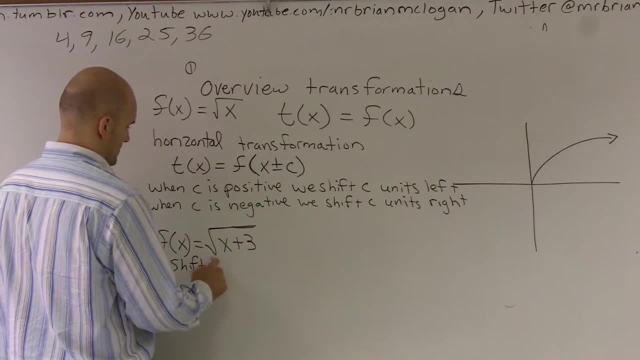 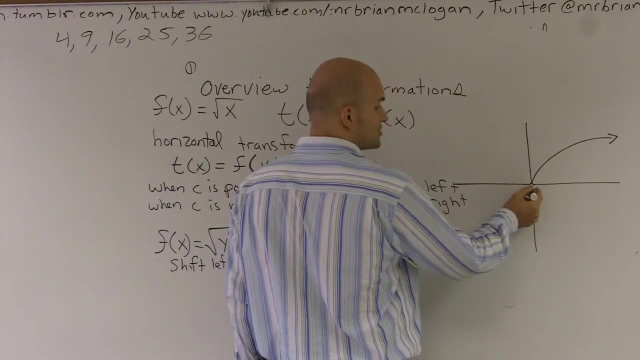 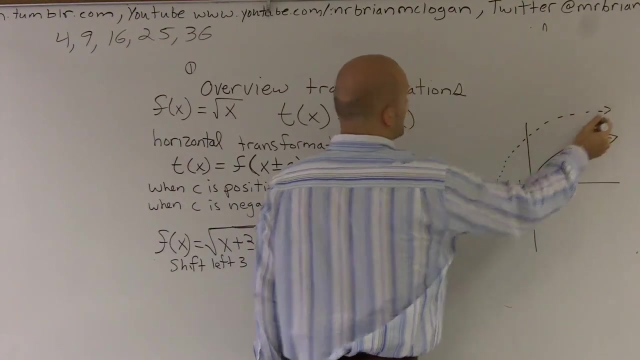 to shift right 3.. So, therefore, if I was going to take my graph, I would just use this point. here's my paragraph. I'd just shift it over 3 units: 1,, 2,, 3. And I'd graph the. 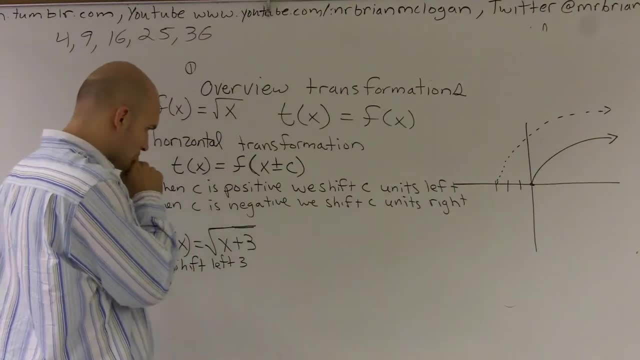 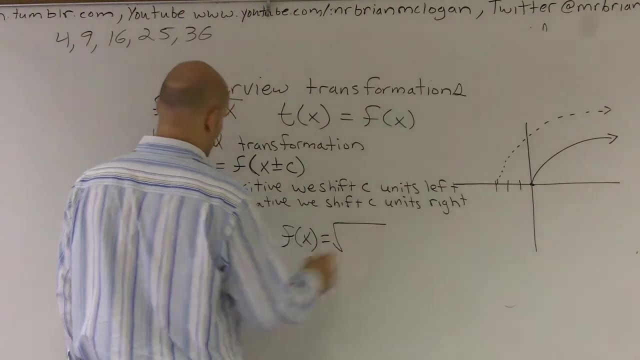 same equation. Furthermore, let's do another one. f of x equals the square root. again, I'll just kind of show you. So I'm going to shift right 3.. So I'm going to shift right 3 and the square root of x plus 3, wrong from it. I'm just going to shift 1. And see when. 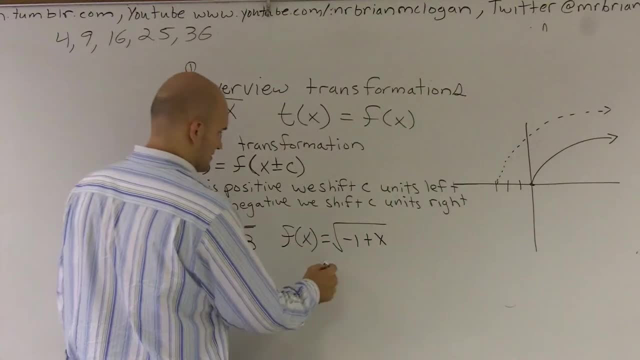 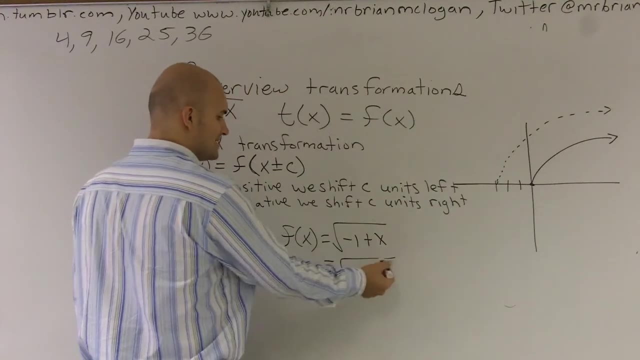 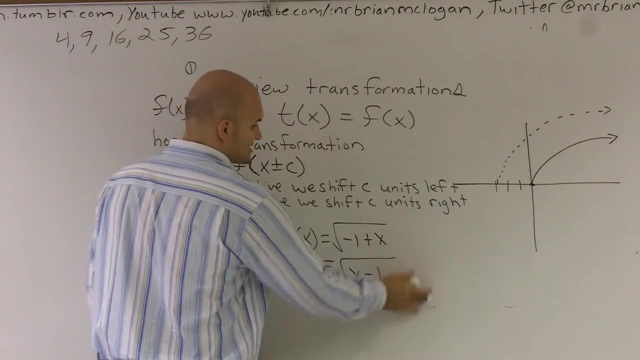 x plus 3 goes around, I'm just going to do the square root and right up the left axis on x. x plus 2 equals negative 3.. If f goes up and down these units, I'm just going to change the length of the fraction. So what I would do is I'm going to take f, I'mchen. 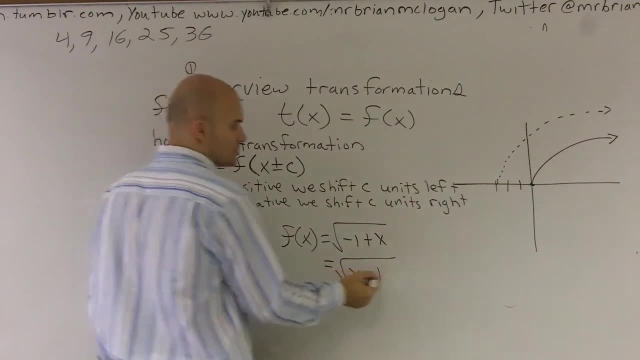 squared up right here. From here I'm actually going to take a second to the square root, and since f goes down, I'm going to just keep going. and 1 minus 1 minus 2 minus 1 minus x equals negative 3.. So what we get is f. if it goes until 1, it will stay in the value. 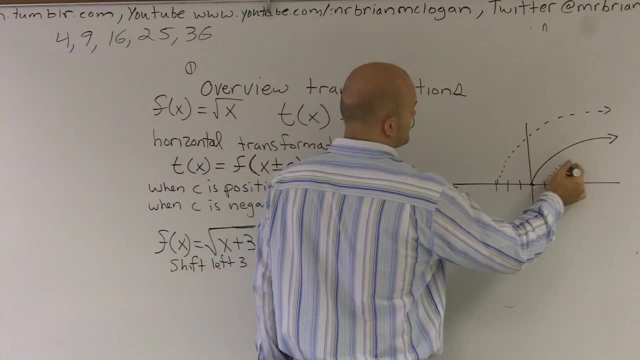 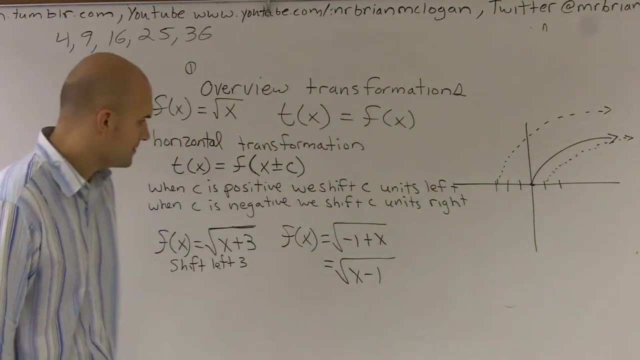 of x. So it's just theاي should be x first. That's the equation for the function dancing Right from here we have our fraction and All right Now like I say: well, how are you getting this true? 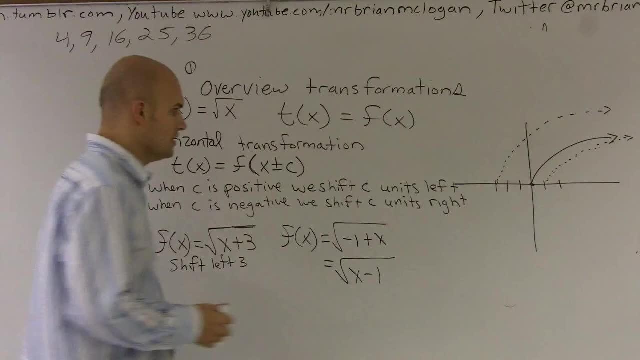 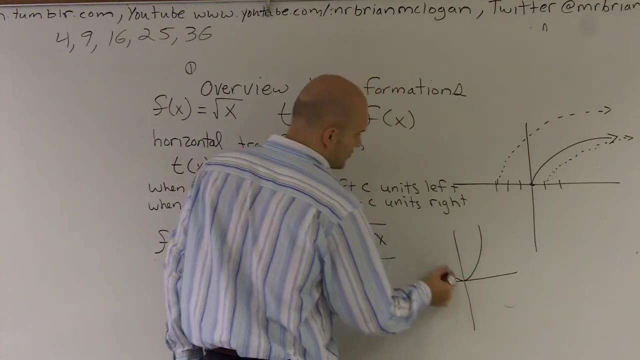 How do you know that it's to the left and to the right? Well, I'll just give you a quick little example. I'll use just a different function, hopefully one you guys are a little bit more familiar with. If we use the function f of x equals x squared. 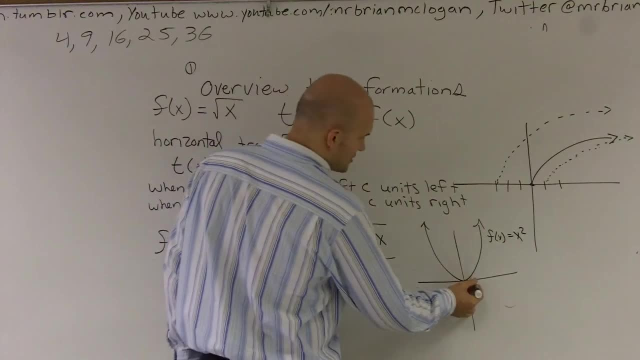 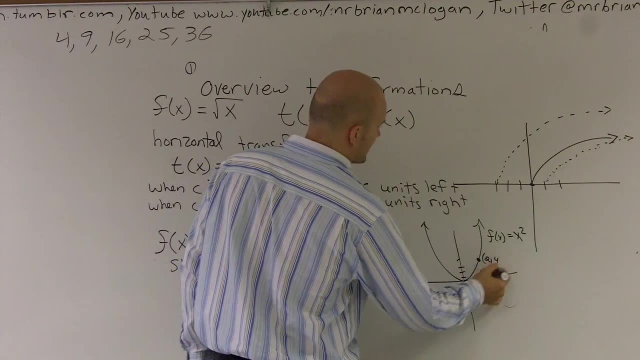 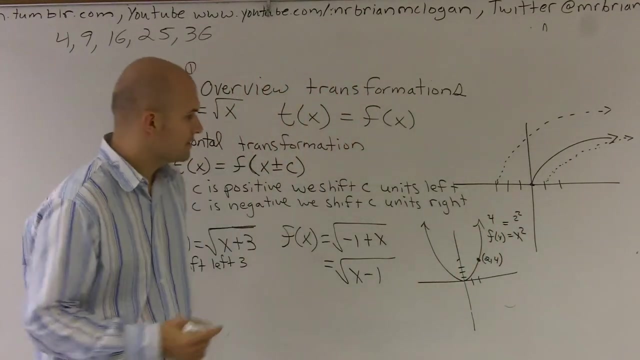 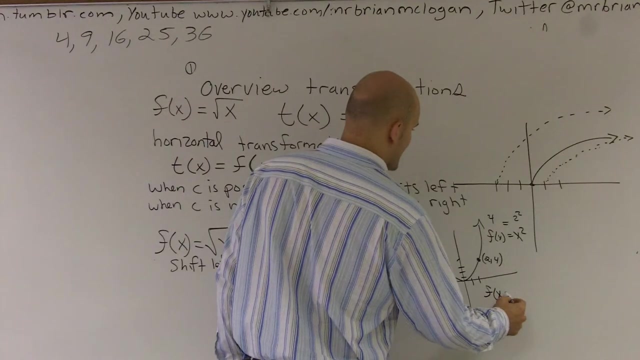 and one thing you guys should know is the point to 4 is on the graph right, Because 2 squared equals 4.. So if I was going to do something and I was going to say, well, how about we did f of x and let's say we now change it to x minus 1.. 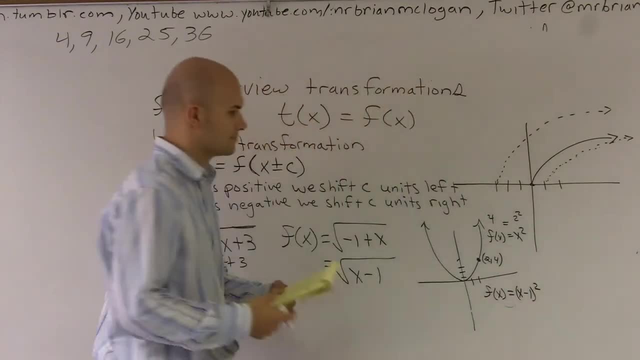 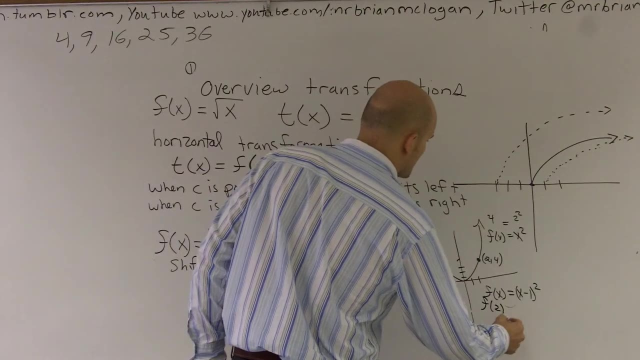 So, therefore, if I was going to now plug in my point and I wanted to find out what is f of 2,, well, you plug in 2, 2 minus 1 is 1, 1 squared is 1.. 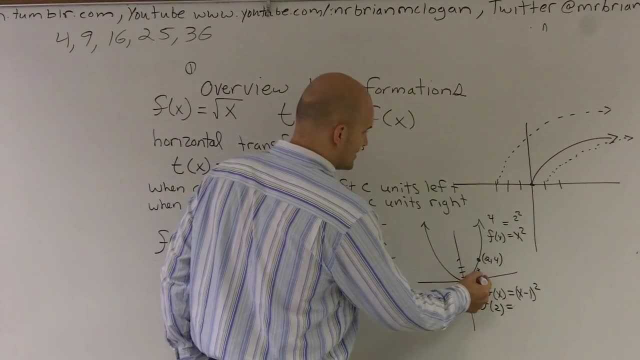 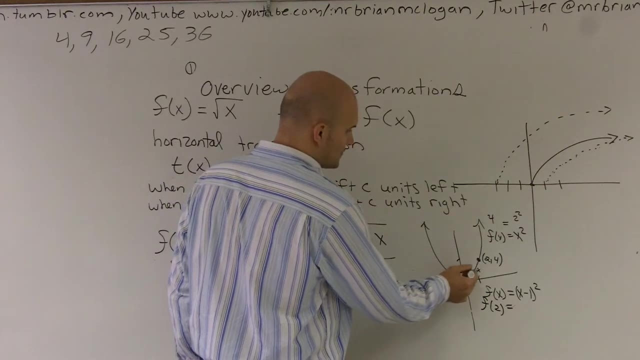 So I'd go over 2, and now my new point would be right there. Well, if you were to shift this graph to the left 1, you think about this. you shifted this whole thing to the left 1,. everything looks the same. 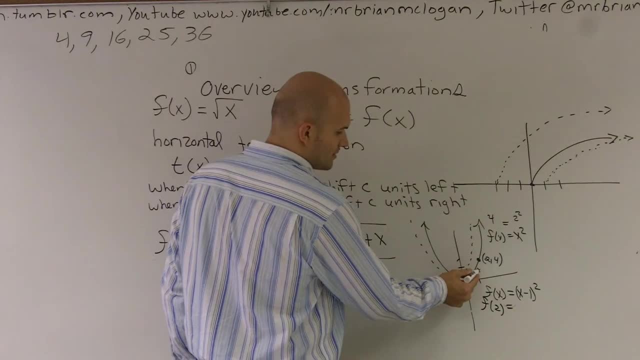